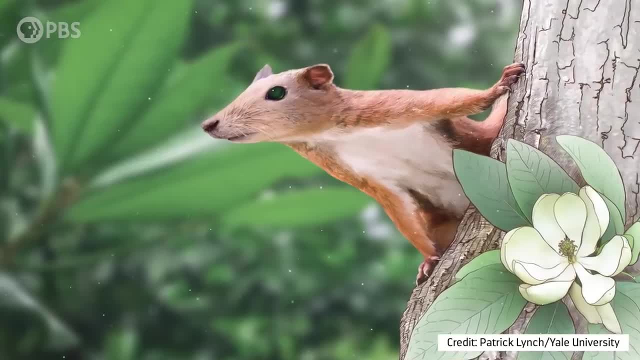 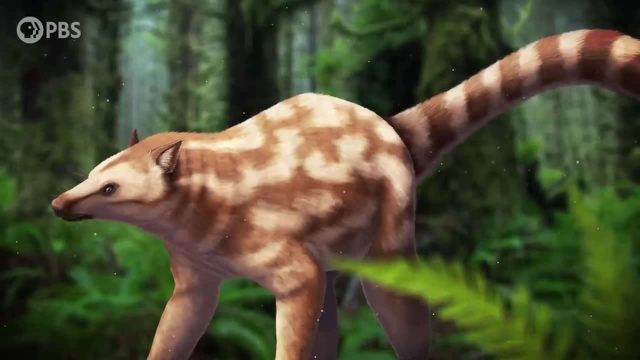 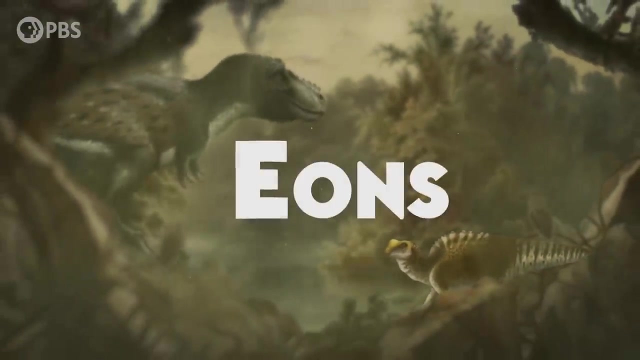 It turns out that the journey towards braininess in mammals was far from straightforward or inevitable. In fact, during one of the most pivotal moments in our evolutionary story, our brains actually shrank relative to our bodies. Now, when thinking about brains, it's important to remember that. 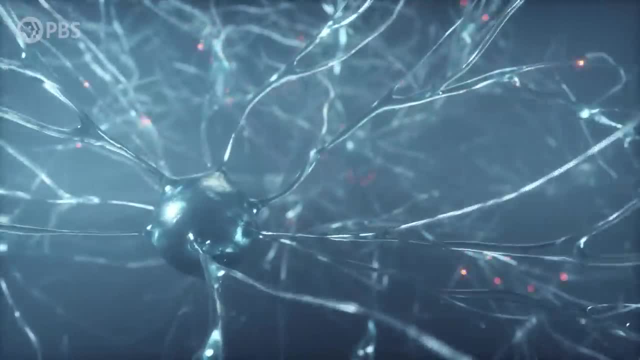 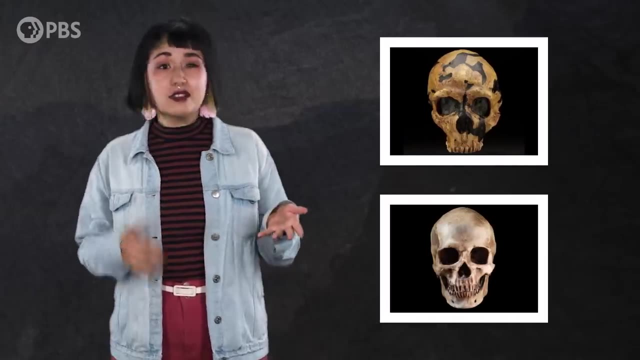 size isn't the only thing that matters. Lots of other factors like structure and density of the neurons also determine how brains work. Take Neanderthals and us modern humans, for example. They had similar-sized brains to us, or even a little bigger in absolute terms. 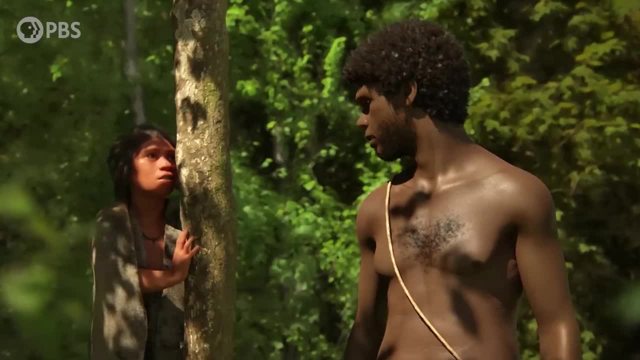 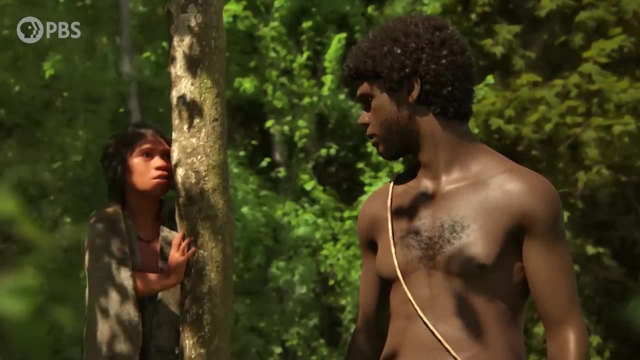 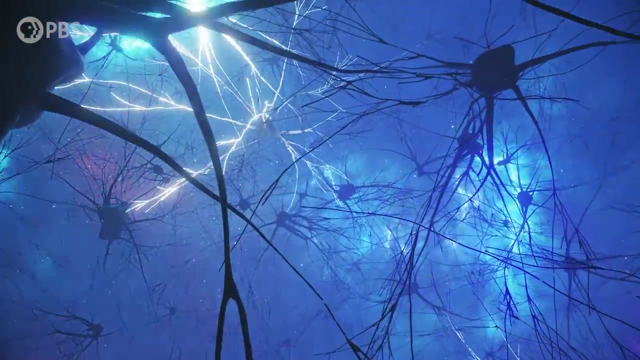 Yet evidence suggests that differences in shape, as well as neuron development and organization, probably led to meaningful cognitive and sensory differences between us and them. But because those aspects of the brain are often hard to examine or compare between species, especially extinct ones, scientists generally just measure what's called encephalization instead, 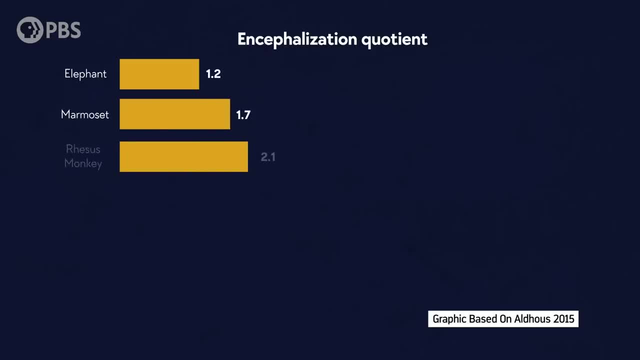 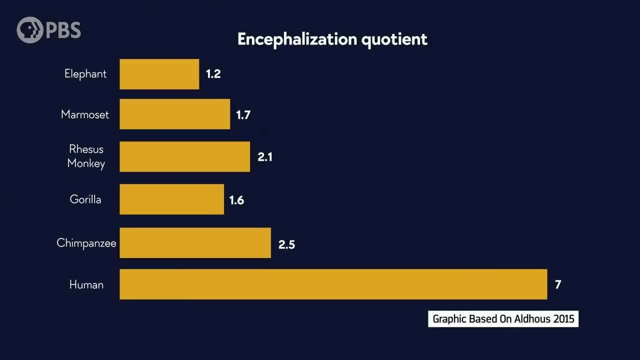 This is essentially a calculation of a specific brain size. It's a calculation of a species' relative brain size based on the ratio between their observed versus expected brain mass for a given body mass. Having a bigger brain than expected by body size alone equals a higher level of encephalization. 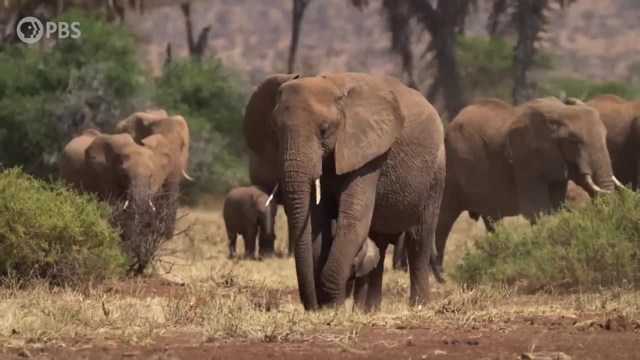 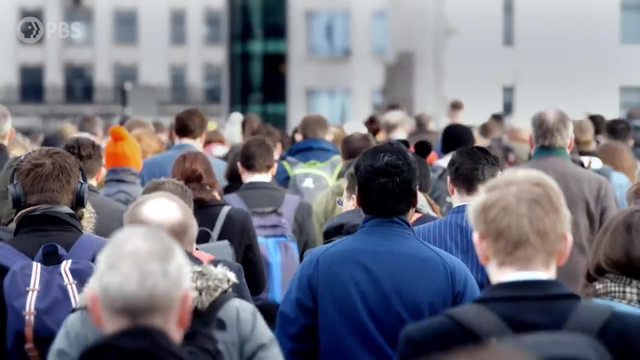 And in vertebrates, encephalization seems to broadly correlate with what we recognize as intelligence. Modern placental mammals are the most encephalized vertebrates, with us humans, the other great apes and dolphins generally coming out on top. 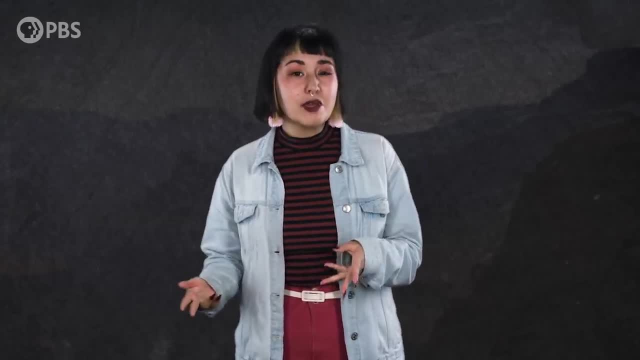 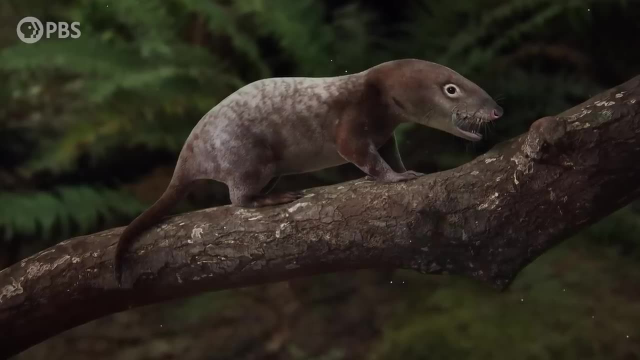 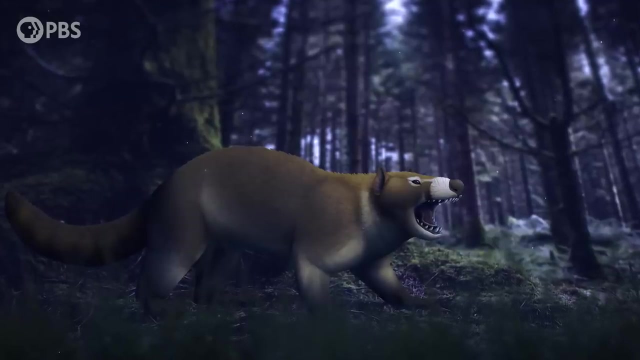 But the evolutionary road mammals took towards becoming so brainy has been pretty mysterious for a while. This is partly because well-preserved fossil skulls from key periods of our evolution have been hard to come by, So we've been left with a lot of unanswered questions like 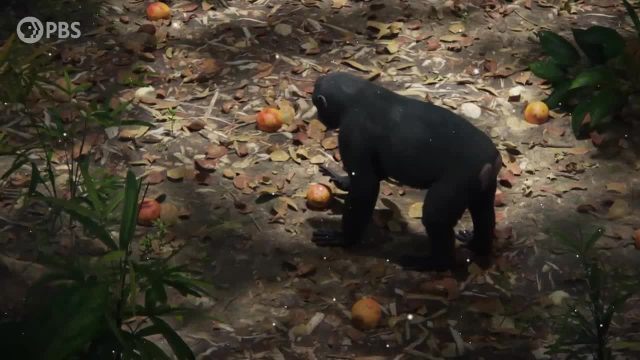 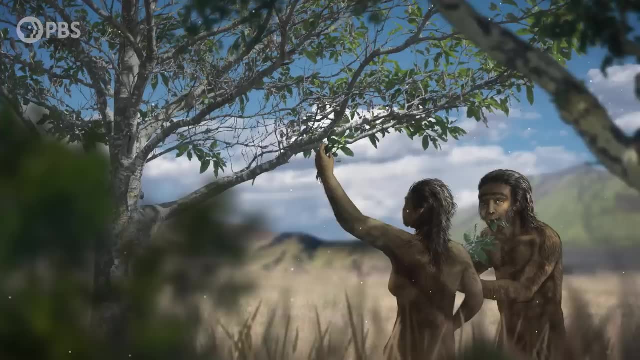 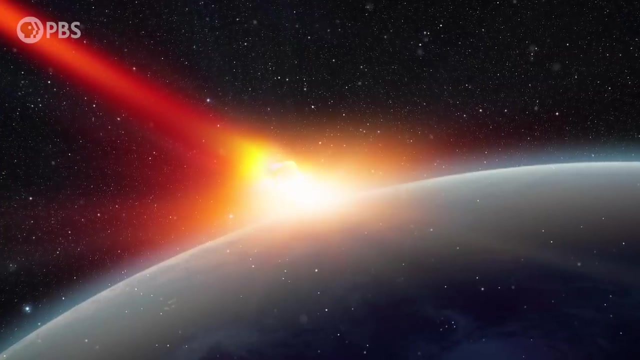 was it a process that started early in our evolution and continued gradually but inevitably over time? What ecological pressures might have driven it, And how was it shaped by key moments in our evolution? We know that the K-Pg extinction, for example, the one that wiped out the non-avian dinosaurs around 66 million years ago. 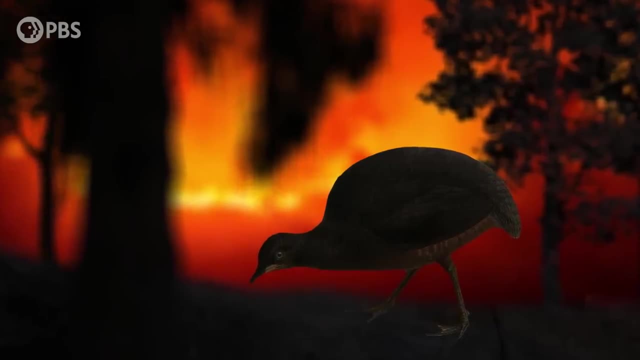 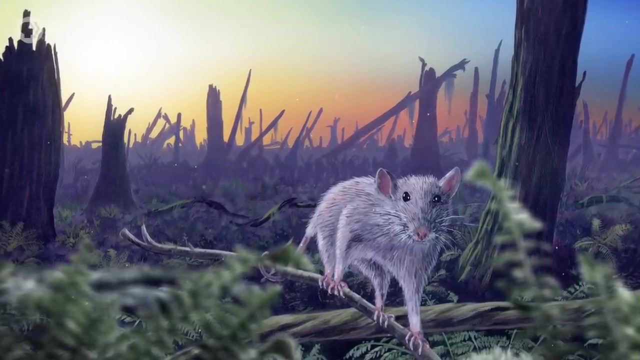 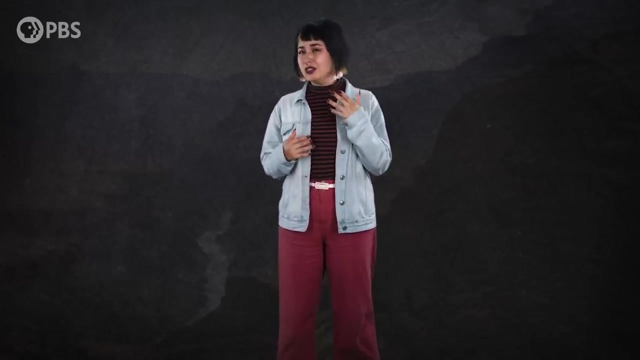 was a major event in the story of our rise, And one common idea was that this period of upheaval may have encouraged the evolution of bigger brains in our ancestors by rewarding ecological street smarts. But ideas like this had actually been really tricky to test. 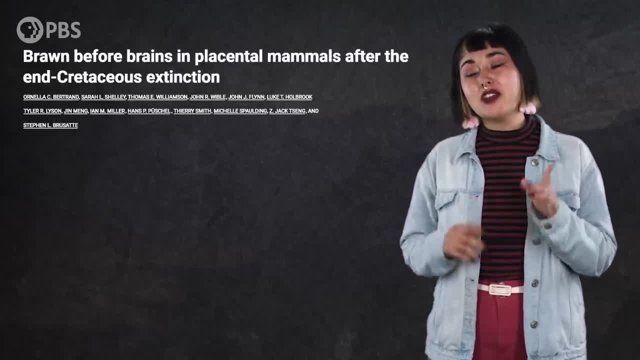 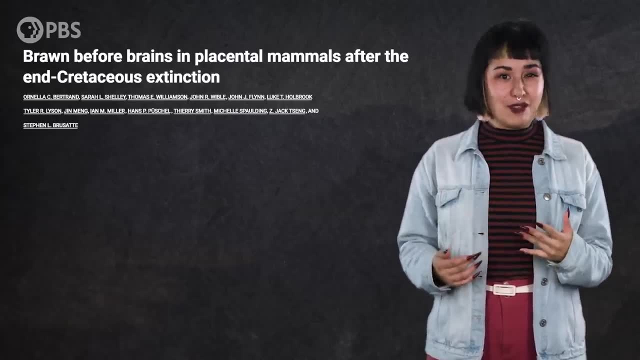 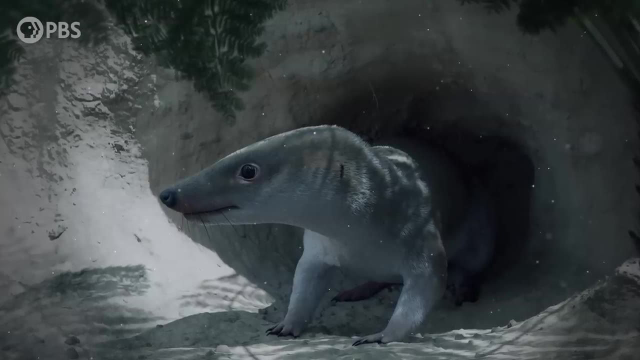 So, in 2022, a team of paleontologists published a new study of brain size data from 124 species, covering much of the evolutionary timeline of mammals From ancient shrew and badger-sized species that lived alongside dinosaurs in the Mesozoic era. 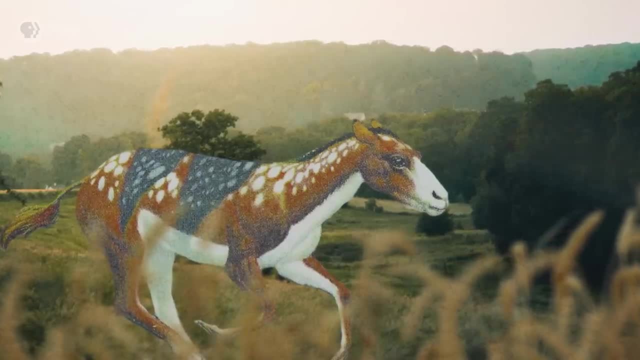 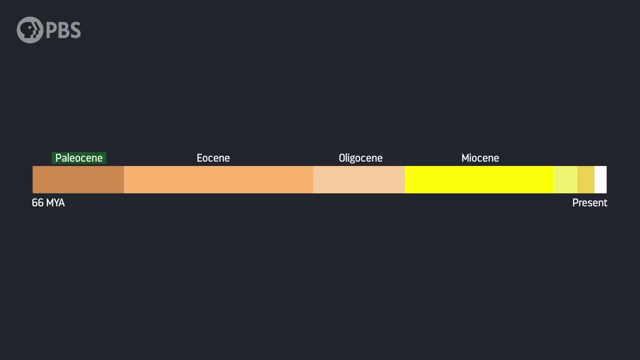 to the first members of many modern groups that emerged in the mid-Cenozoic era And they high-resolution CT scanned some newly discovered fossils from the crucial prehistoric period of the Mesozoic era And they found that the K-Pg extinction was the window in the middle of this timeline. 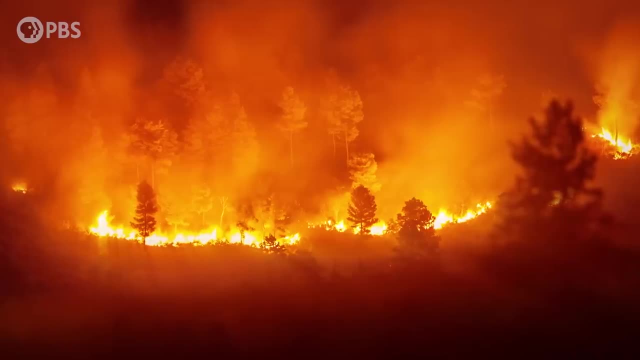 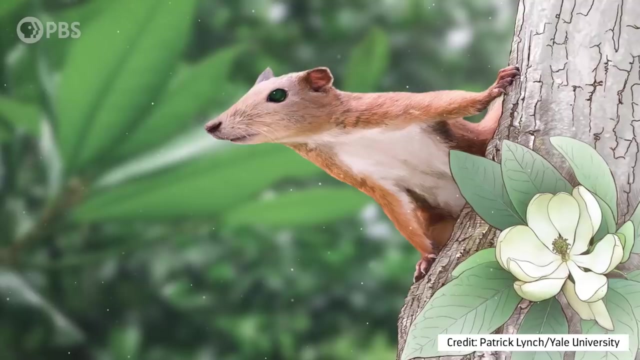 The Paleocene Epoch, The time period that includes the direct aftermath of the K-Pg extinction, But instead of the intertwined chaos and opportunity of that situation, rewarding mammals that could problem-solve and adapt, thus pushing us inevitably towards ever-bigger brains, 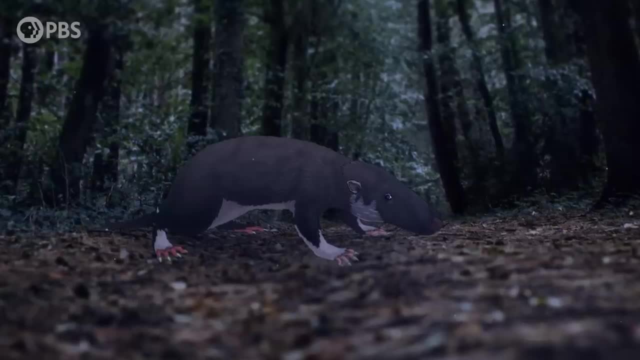 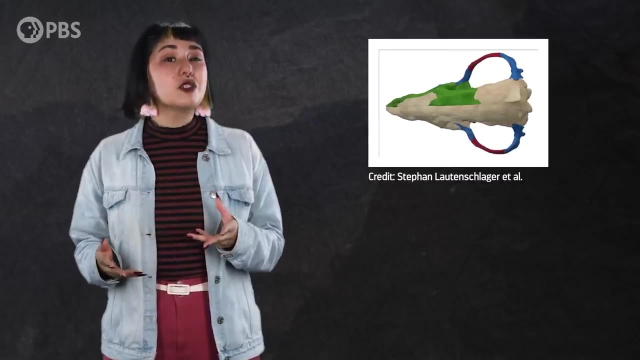 the data told the complete opposite story. See mammals from the end of the Mesozoic: small-bodied and small-brained. Their encephalization was much lower than that of modern mammals, although the proportion of their brain responsible for smell was higher. 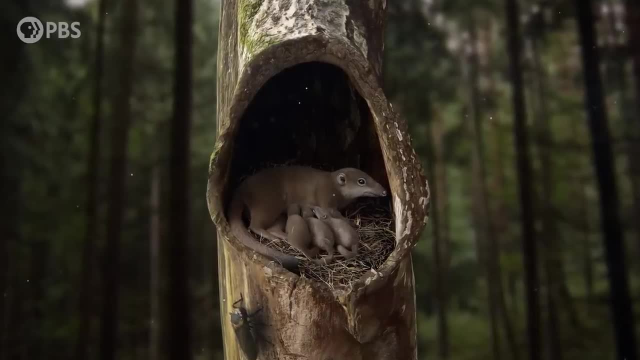 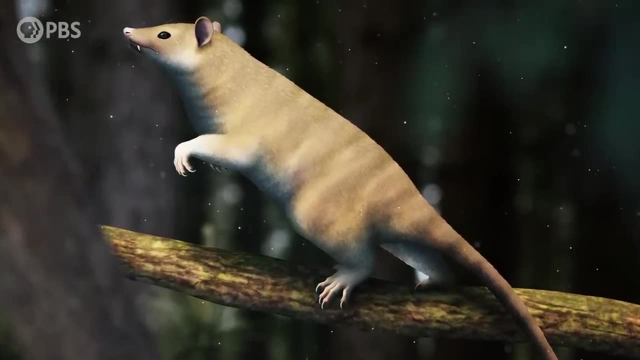 Otherwise, though, their sensory capabilities and overall intelligence were probably nothing to write home about. Yet mammals that came after them in the Paleocene in the wake of the K-Pg didn't increase in relative brain size from this low base level, it turns out. They shrank even more as the planet recovered. Now, this isn't to say that their brains shrank in absolute terms compared to their Mesozoic ancestors and relatives. They actually got bigger, But mammal body sizes grew at a much faster rate over the 10 million years post-K-Pg. 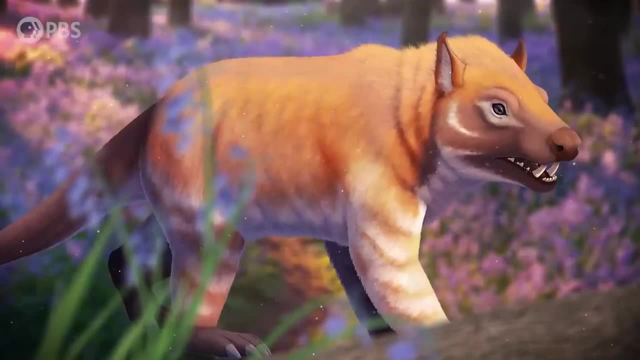 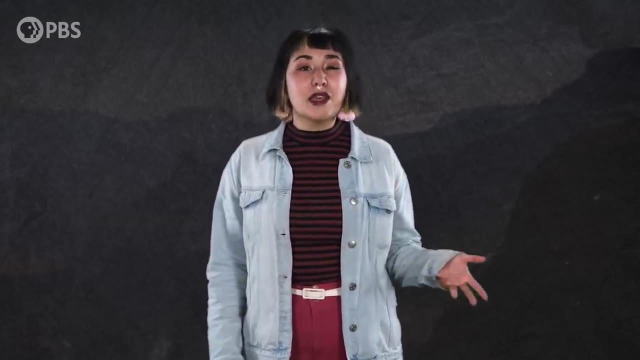 which left them less encephalized overall than both later and earlier mammals. So what happened here? Well, the answer goes back to one of the most basic things we know about evolution. It's a game of constant trade-offs and in some ecological situations, 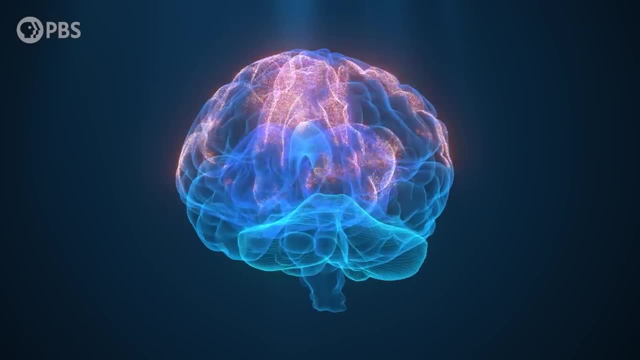 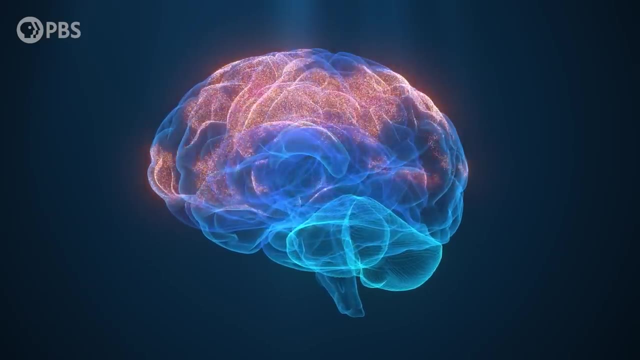 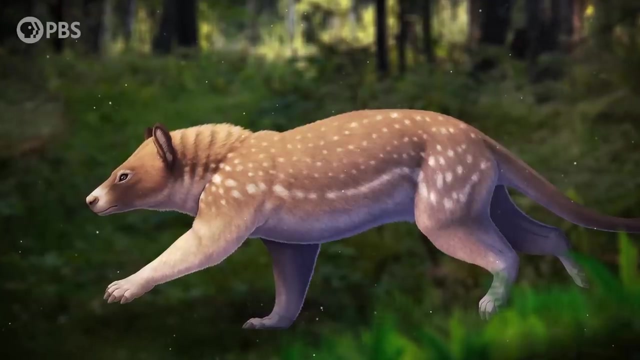 being smarter isn't an advantage. Having a big, powerful brain is really expensive in terms of energy requirements. Pound for pound, brain tissue uses almost an order of magnitude more energy than other body tissues, Despite providing greater cognitive, behavioral and sensory capabilities. in some situations, having to fuel a big brain can reduce an organism's ability to survive and reproduce. And the immediate aftermath, The aftermath of the K-Pg- seems to have been one of those times, With the demise of the non-avian dinosaurs. 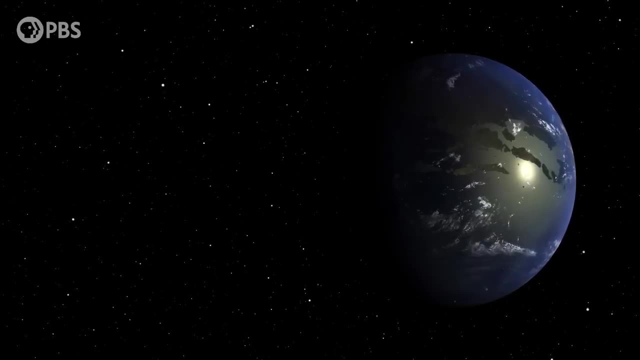 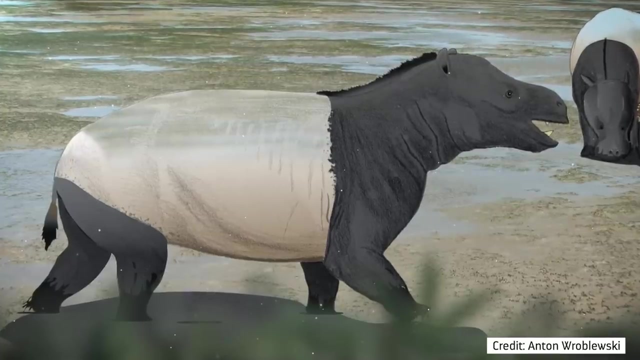 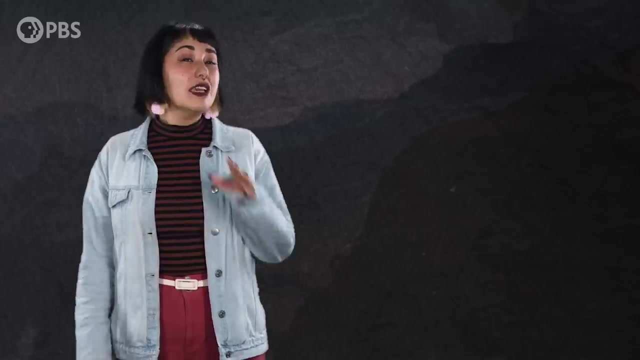 mammals that survived the catastrophe were faced with an opportunity that would define the rest of the Cenozoic and usher in the Age of Mammals. As ecosystems recovered and new food webs emerged. previously unavailable ecological niches were now open to them. 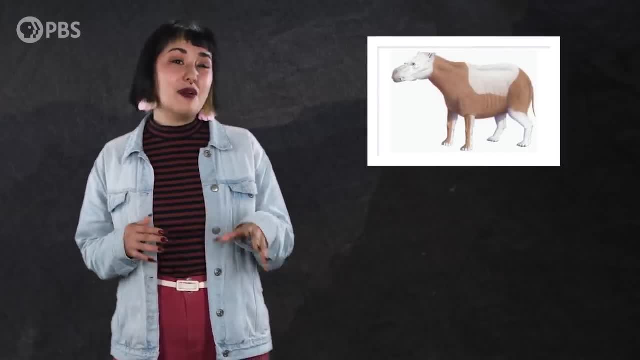 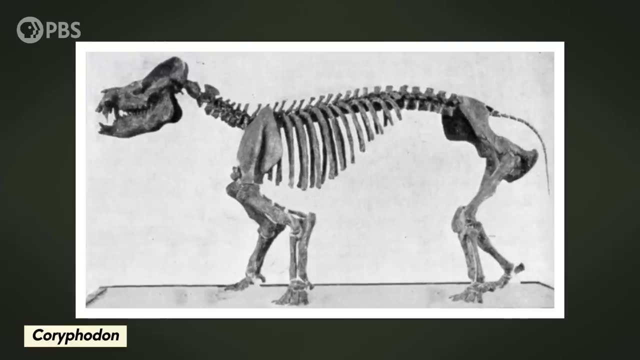 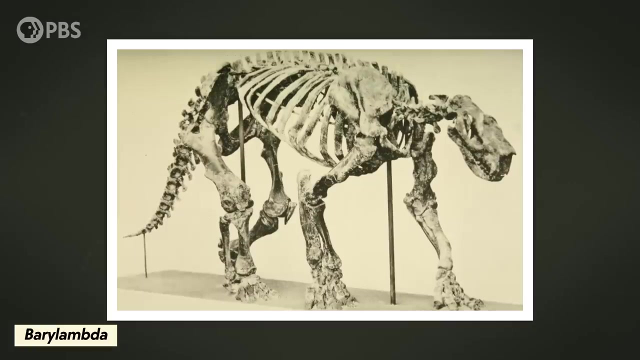 Take the pantodonts, for example, an ancient, extinct group of medium- and large-sized herbivorous mammals with proportionally tiny skulls. They included some of the earliest recorded Paleocene mammals to get bigger from the much smaller Mesozoic ancestors, filling gaps in the ecosystem that had previously been occupied by 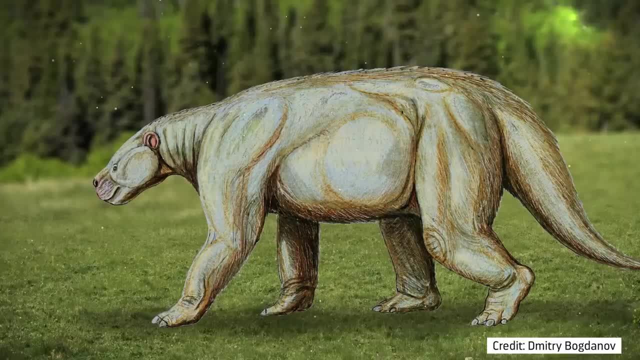 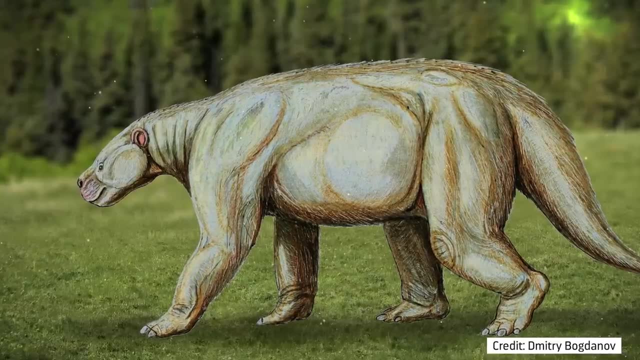 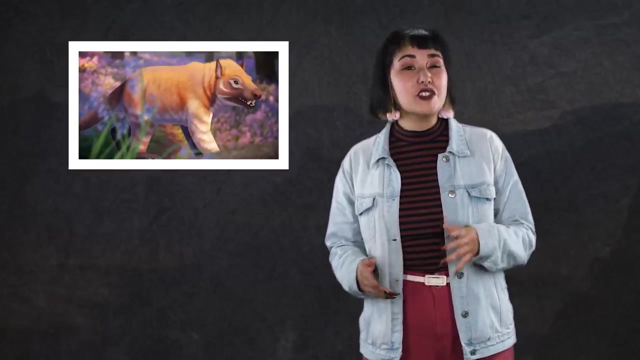 medium- and large-sized herbivorous dinosaurs, And it seems that getting brawny rather than brainy was quite literally the bigger priority for radiating into those niches. The CT scanning the researchers did also revealed how the size and shape of different brain regions changed over this period. 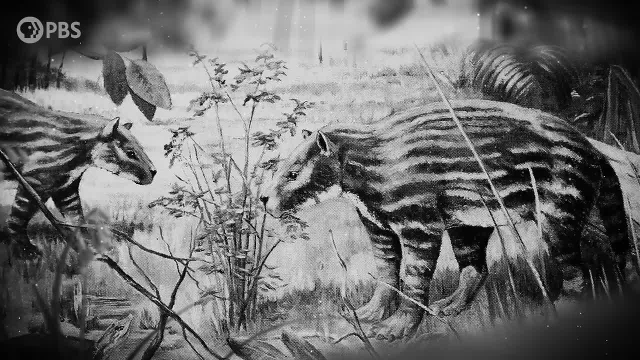 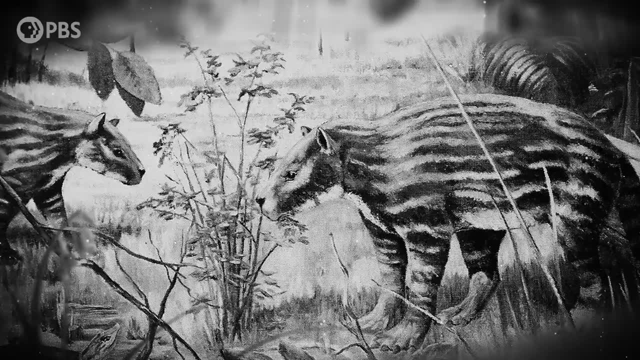 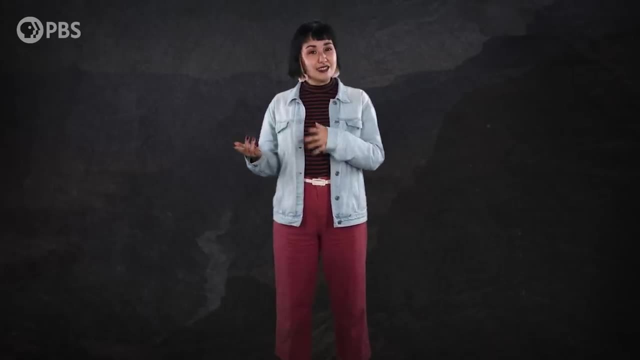 Or more specifically, how little they changed, Because the brains of the pantodonts and other Paleocene mammals grew only as much as necessary to control their larger bodies, which scaled up at a much faster rate. So during this time the increase in size did not include any major changes in the brain's structure. 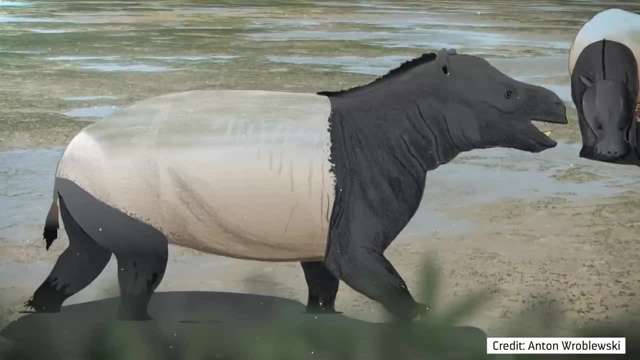 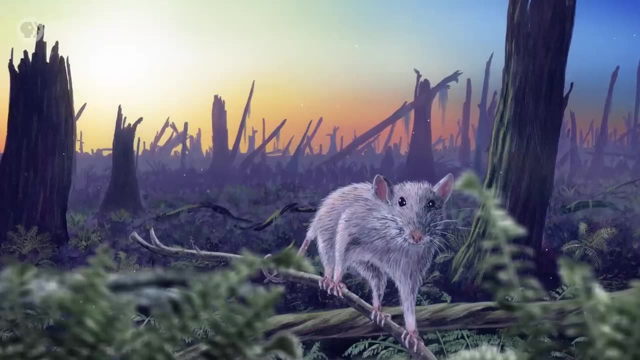 or the addition of new features. This left them with proportionally smaller brains and no new sensory or cognitive regions compared to Mesozoic mammals. In this new post-apocalyptic world with lots of empty niches and little competition, thinking was overrated. 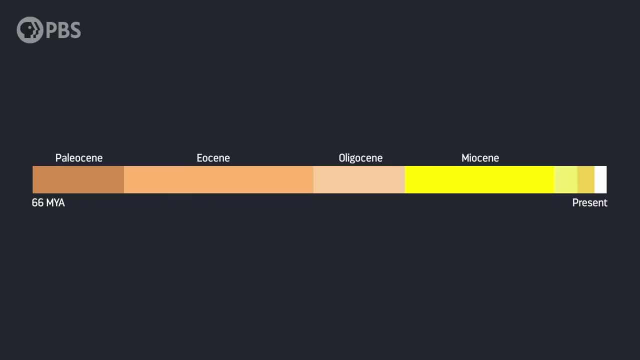 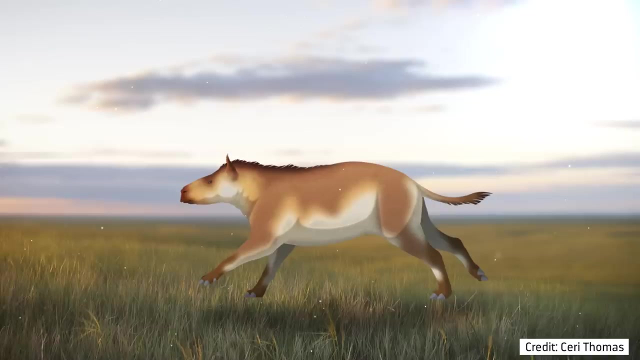 In fact, the researchers found that mammal brains only really started a catch-up with their bodies as the Paleocene gave way to the Eocene epoch around 56 million years ago. Multiple mammal lineages independently experienced shifts towards much greater encephalization around this time, with body growth slowing down and brain growth picking up. 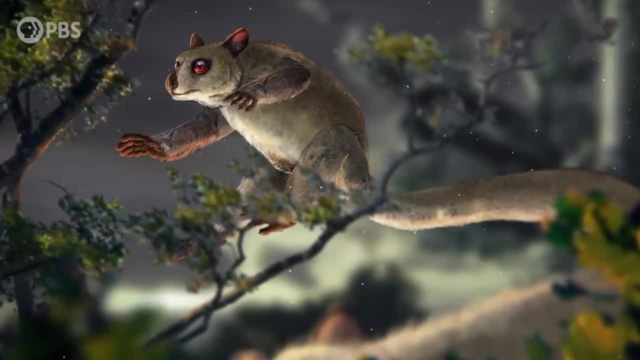 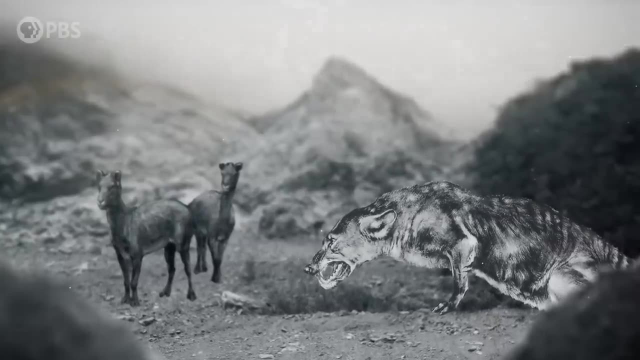 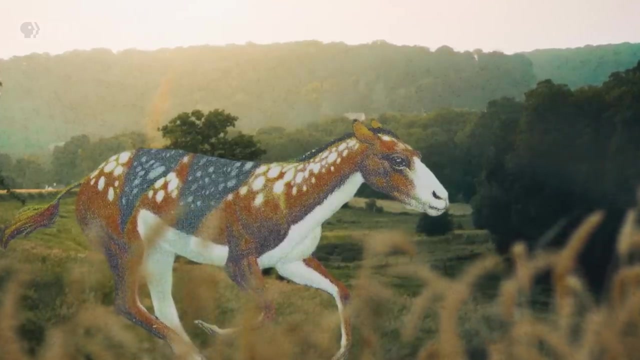 And that was probably a result of ecosystems fully recovering by this point and reaching a high level of saturation. In such rich and competitive ecosystems, bulking up was no longer enough to secure success. This new world instead rewarded the ability to think on your feet. 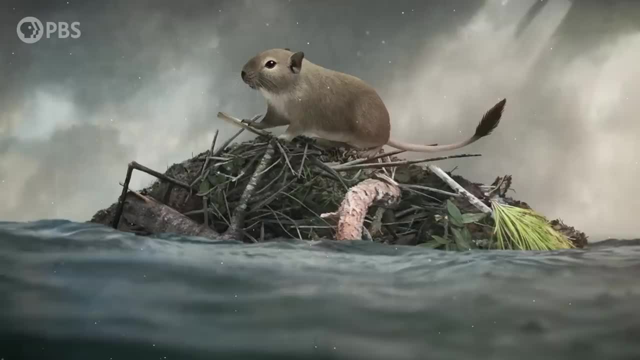 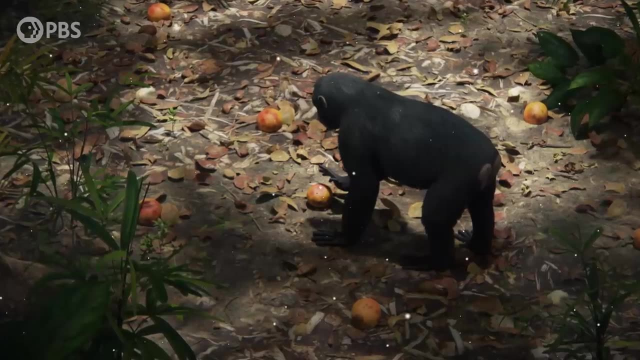 Or paws Hooves. So being brainy finally became amazing. It was a major advantage for many mammal lineages, simultaneously including ours. The researchers found that encephalization really took off in certain early mammals that emerged around this time. 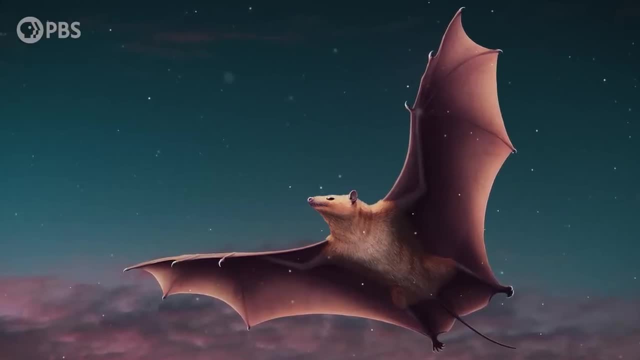 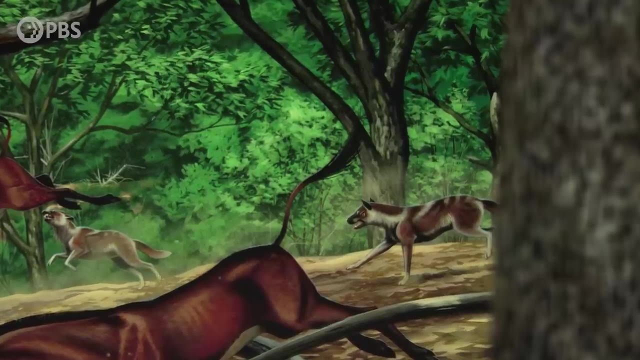 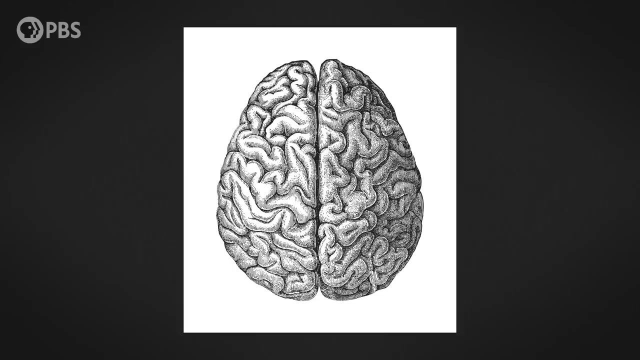 The ones that were ancient members of living groups that are still around today. They included the first horses, whales, dogs, bats and primates, which all saw huge increases in encephalization compared to both their Paleocene and Mesozoic relatives. 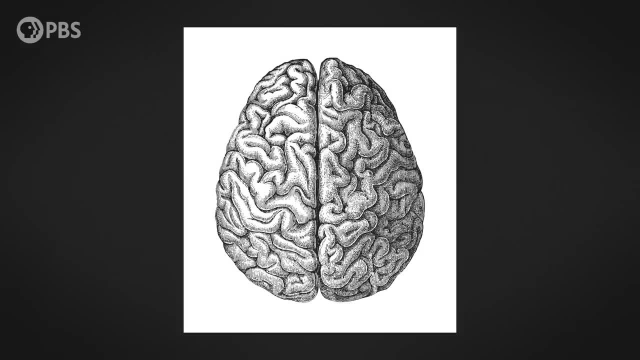 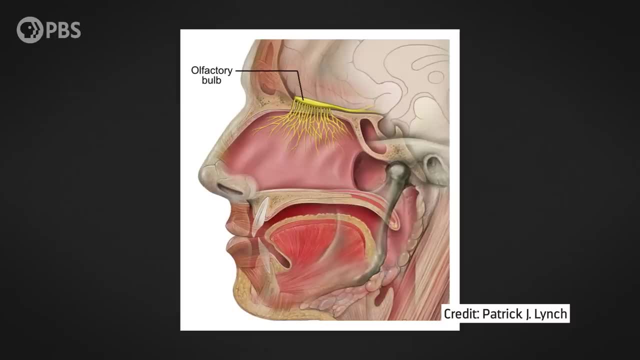 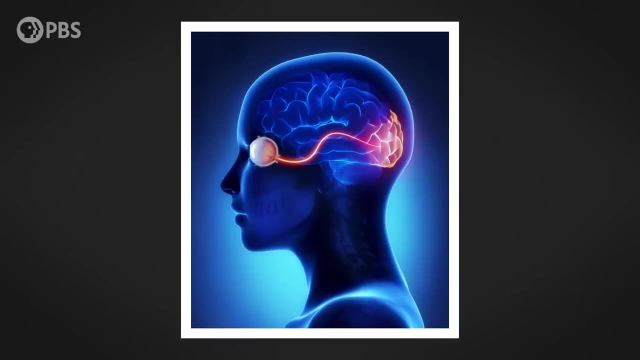 Their brains didn't just scale up, they changed radically in structure too. Their olfactory bulbs, which are responsible for sense of smell, became proportionally much smaller, And the regions of their brains involved in vision, eye movement and balance became proportionally larger, along with the neocortex, 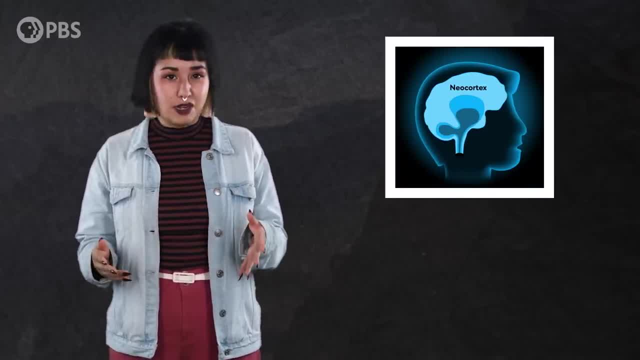 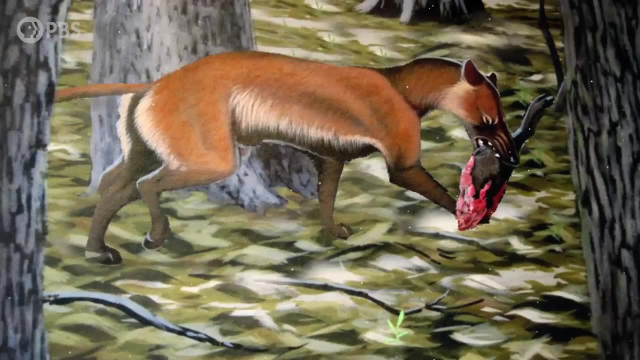 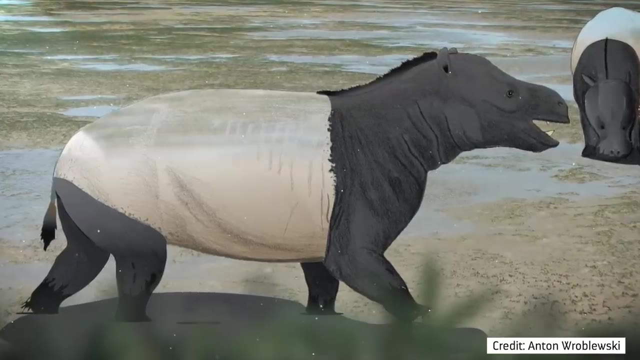 This is a highly complex outer region that helps to integrate processes and anticipate sensory information, and is responsible for higher-order thinking. Growth in these regions gave those more encephalized mammals the edge over more ancient small-brained critters like the pantodonts, who still relied mostly on smell. 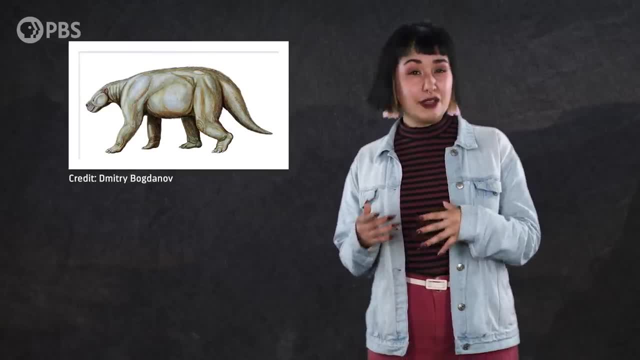 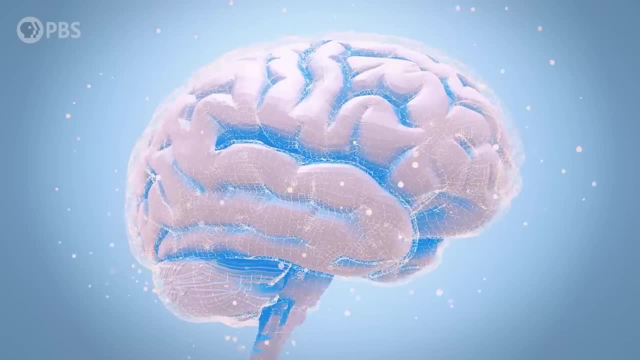 And that might be a big part of what led to those ancient mammal lineages declining over the Eocene epoch as the newer groups radiated and outcompeted them. So, when all is said and done, maybe we mammals should be proud of our big, complex brains. 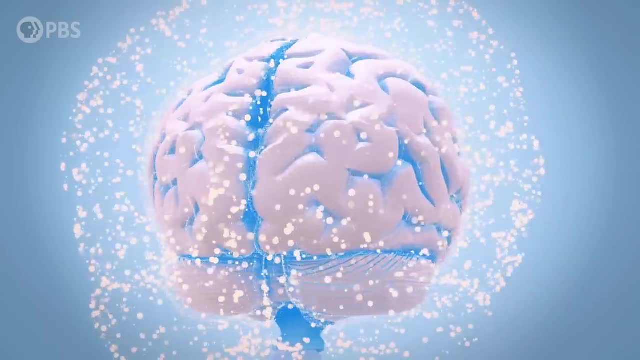 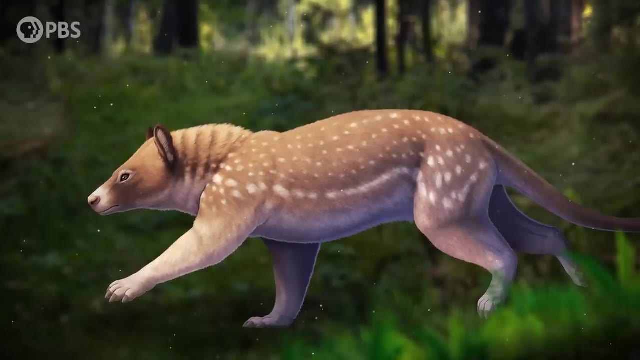 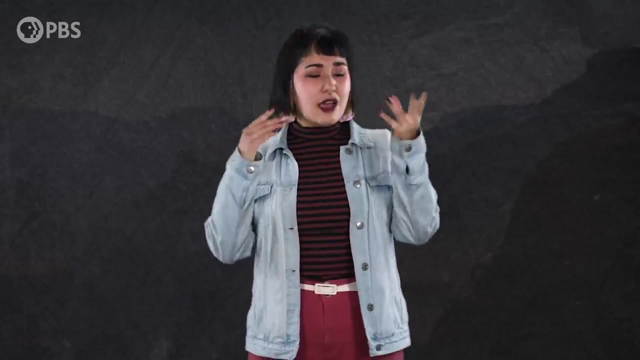 as they've served us well over our more recent evolution. But if you trace our story back far enough, they actually dropped a place on our list of evolutionary priorities, And at a pivotal moment too. And all this shows that there's no inevitable linear evolutionary progression towards bigger. 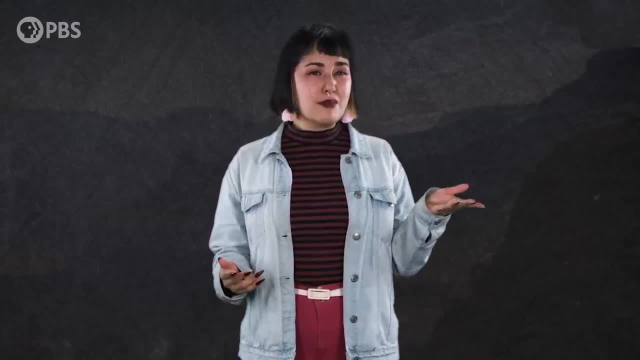 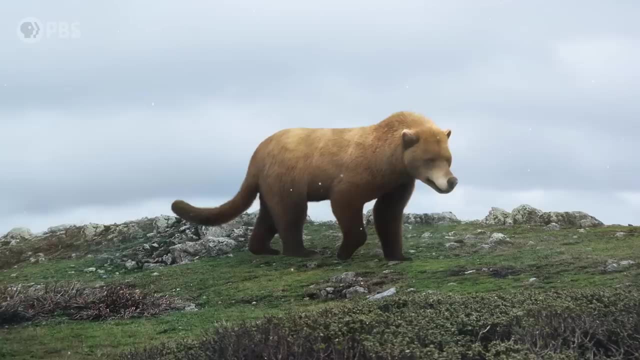 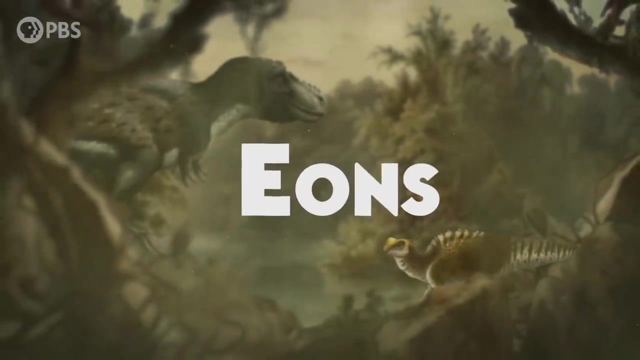 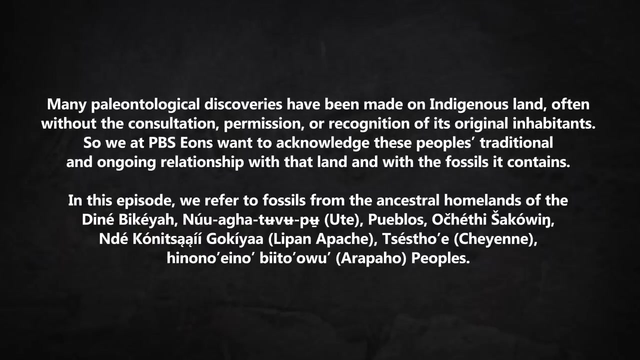 brains and higher intelligence, Or any other traits for that matter. Evolution is about trade-offs, contingency and ecological context, And that's something we should always bear in mind. That's what we're ergません. Thank you to Brilliant for supporting PBS. 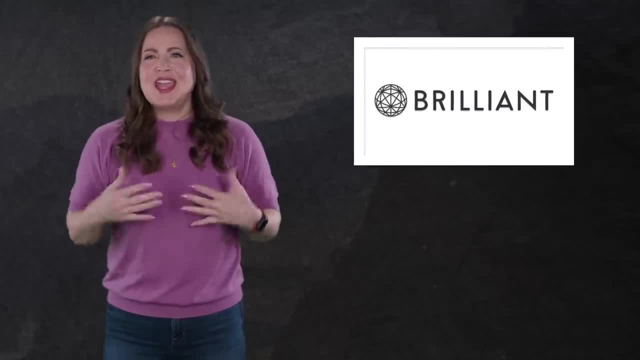 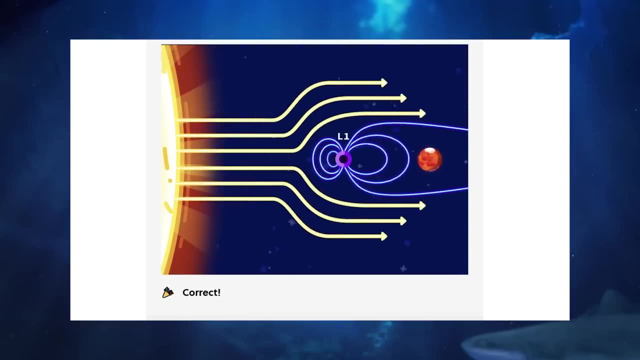 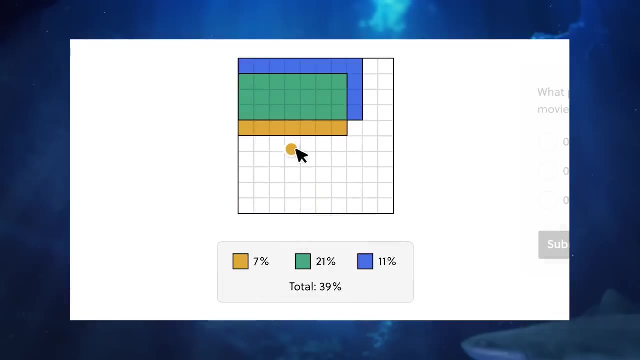 Brilliant is an online learning platform for STEM with hands-on interactive lessons. Brilliant is for curious learners, both young and old, professional and inexperienced. Brilliant courses teach you how to train and navigate better. teach you how to think via interactive lessons and problem-solving activities or exercises. 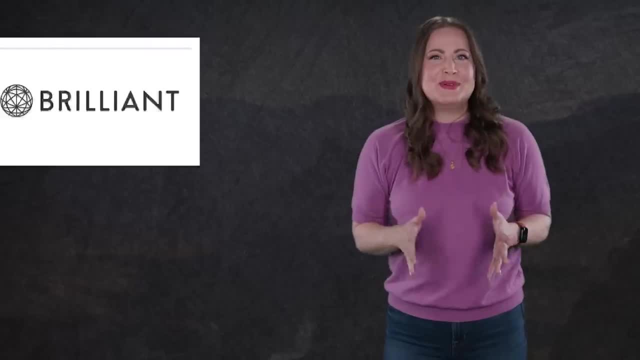 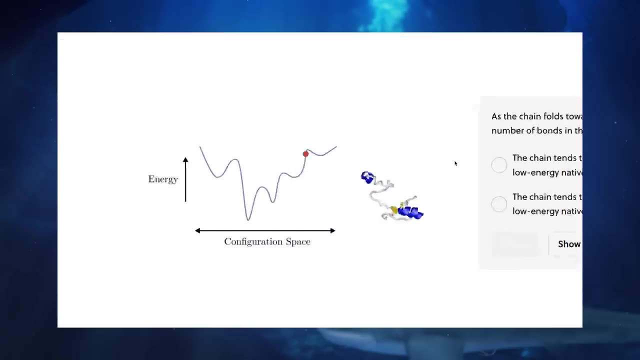 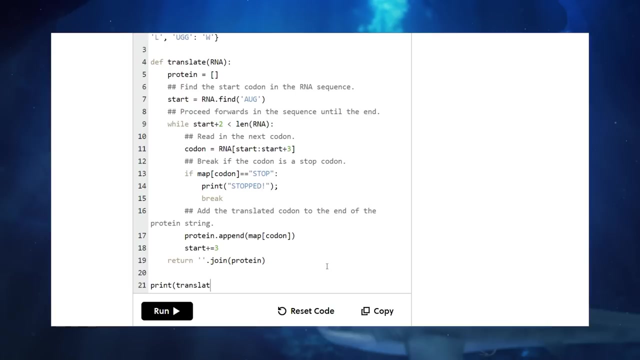 and solve problems with interactive lessons in STEM, For example, Computational Biology, was written in collaboration with quantitative biologists and biophysicists. This course merges the algorithmic thinking of computer scientists with the problem-solving approach of physics to address the problems of biology. 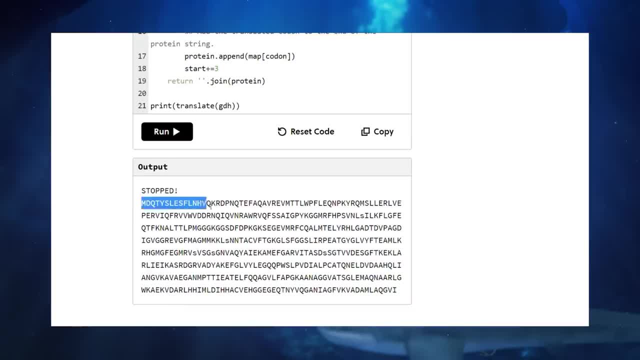 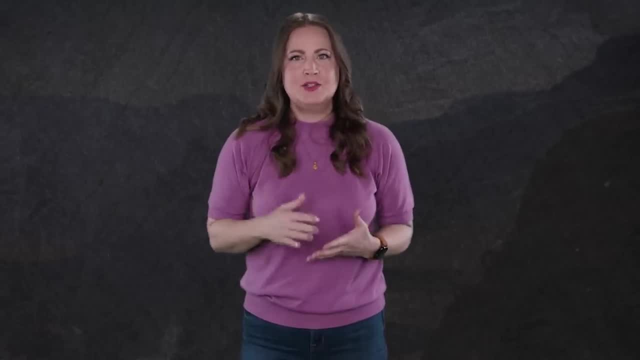 Since the year 2000, an ocean of sequencing data has emerged that allows us to ask new questions. Here you'll develop an intuition for a selection of foundational problems in Computational Biology, like genome reconstruction, sequence alignment and building phylogenetic trees. 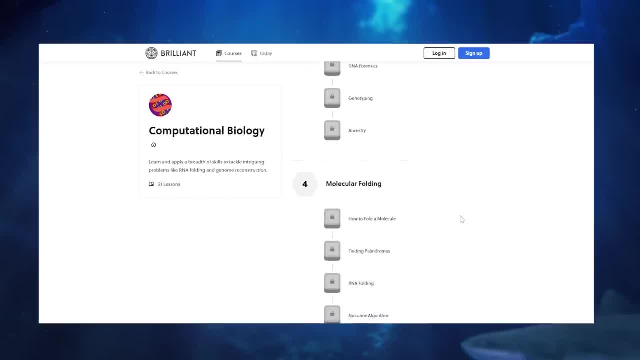 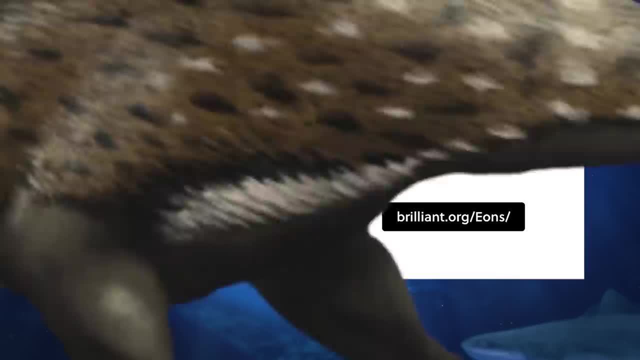 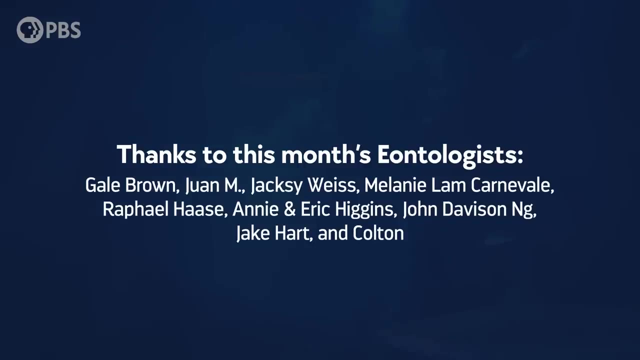 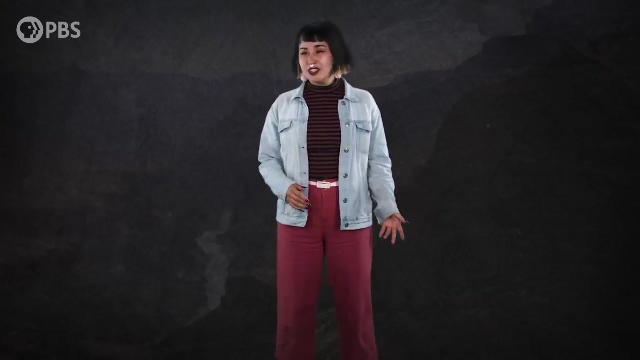 to look at evolutionary relationships. You'll also address certain problems of molecular biology like RNA folding. To learn more about Brilliant, go to Brilliantorg slash eons. Thanks to this month's Brainy Eon Talk, By becoming an eonite at patreoncom slash eons, you can get fun perks like submitting. 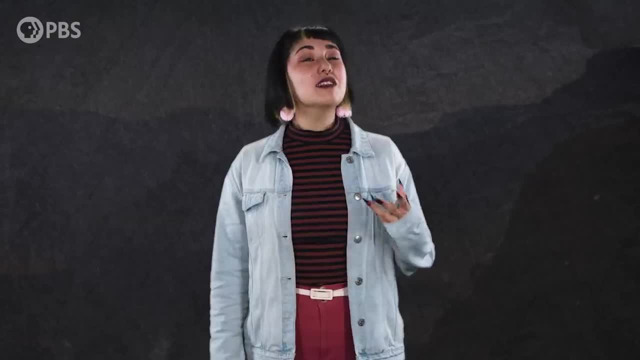 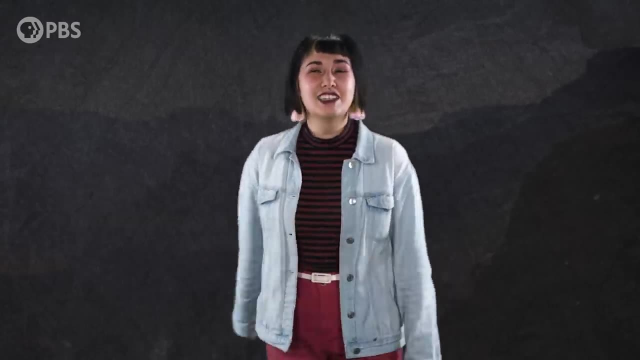 a joke for us to read. Here's one from Todd What's the most polite prehistoric reptile, A PLEASIOSAUR, And, as always, thanks for joining me in the Adam Lowe Studio. Subscribe to my YouTube channel and I'll see you in the next video. 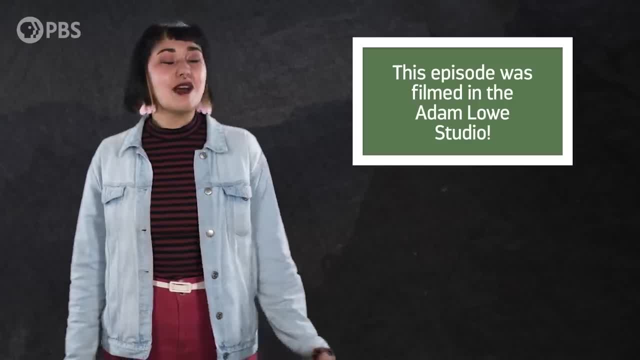 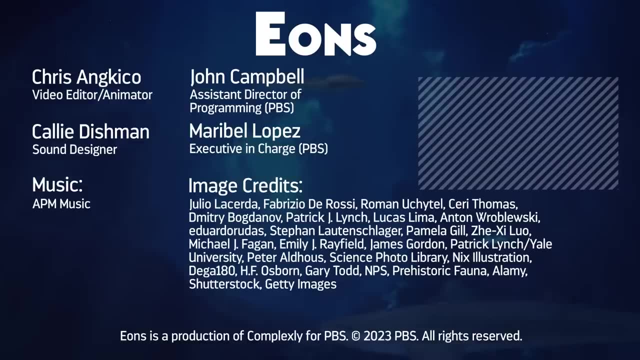 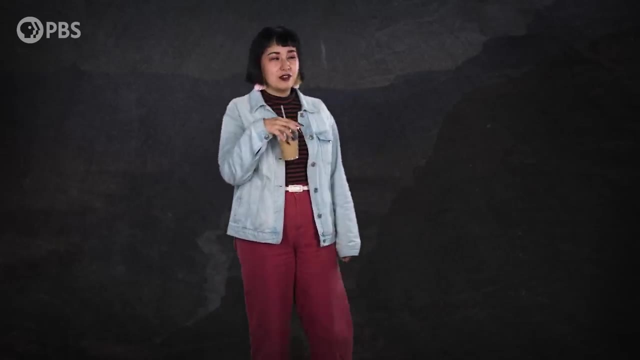 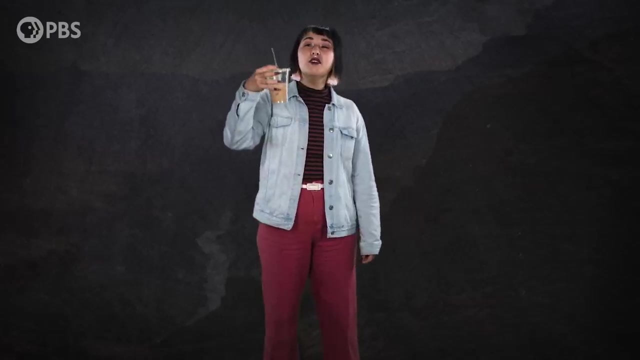 Bye. Subscribe at youtubecom. slash eons for more Fabulous Fossils. I'm in equilibrium with the outside world right now. It's cold outside. I'm cold outside.